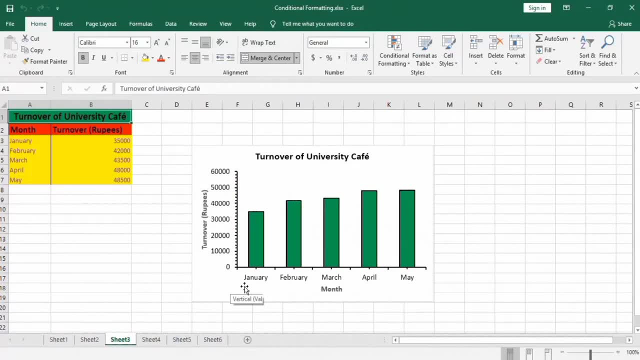 In this video you will learn how you can change these x-axis values, For example. currently, these are the months which are shown here. I will change these months with years, So let's learn how to clear this one Before that. if you are interested to change this minimum and maximum values of y-axis, or the major or minor unit change, you can watch my other video. I will provide the link in description. So let's start this tutorial. 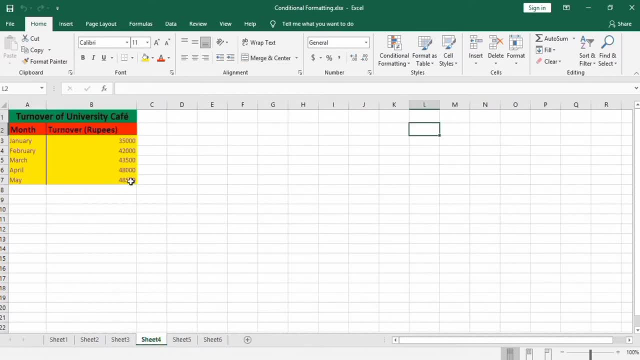 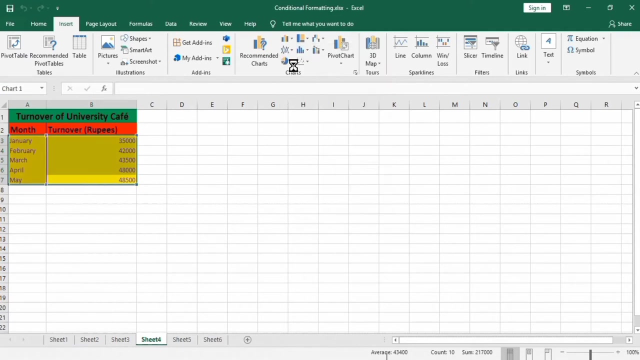 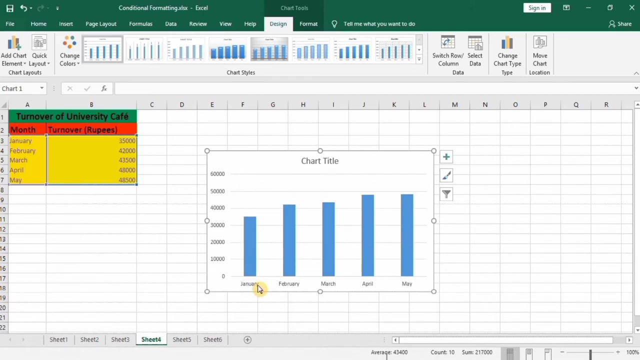 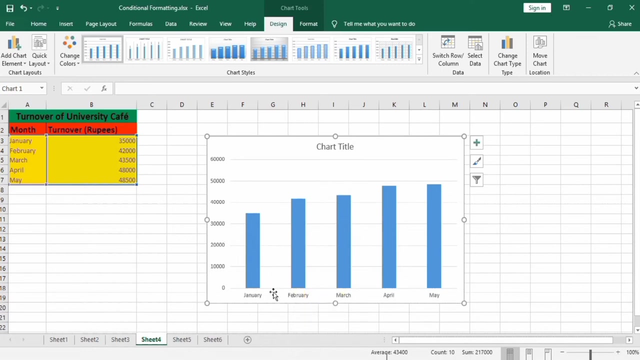 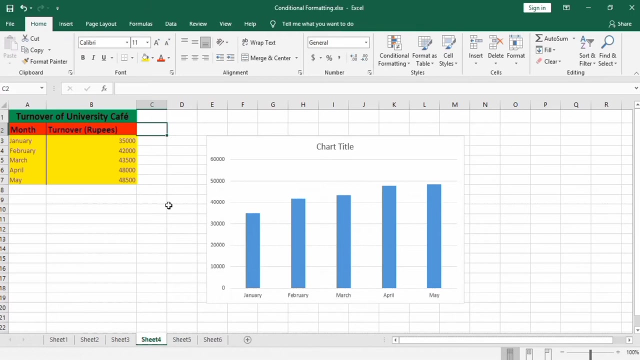 Firstly, select this data to generate a graph. Go to insert tab and select clustered column chart. Remember that you can follow the similar procedure for line graph to change the x-axis of line graph. Firstly, I will resize it. I will not format this graph. If you are interested in formatting of this graph, you can watch the other video. Select this axis firstly, and before that I will generate a separate column. I want to display year here, So I will write year and 2010.. 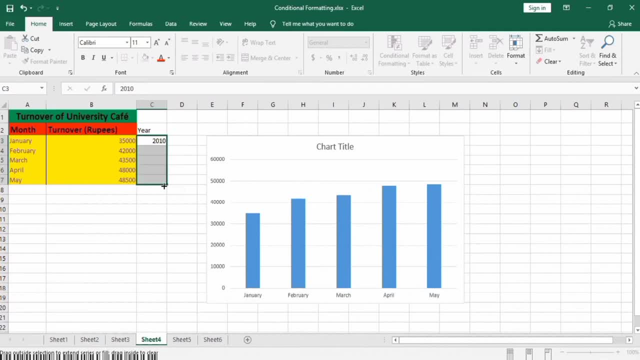 And I will select field series option. So these are the years which I want to display here. Now I select this axis. You can see here that x-axis is selected. now Right click on it And here you will find the option of select data. Click on this option. 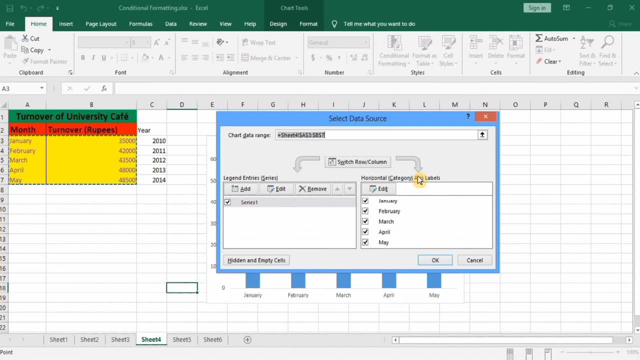 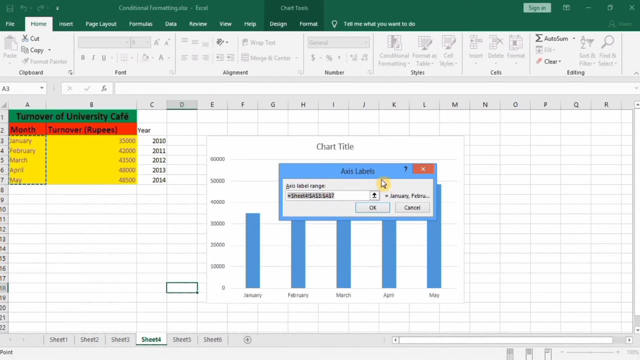 Now in horizontal axis tools, click on this Edit option and a dialog box appear like this. Now you will select the range of here. Now for the x-axis. I want to show this, so I will select this one. Firstly, I will remove all the entered data, then select this. You can see here that this data is selected. So here below I will add the second field here. So you can see here on the end, I have added all my selected fields And this is format. 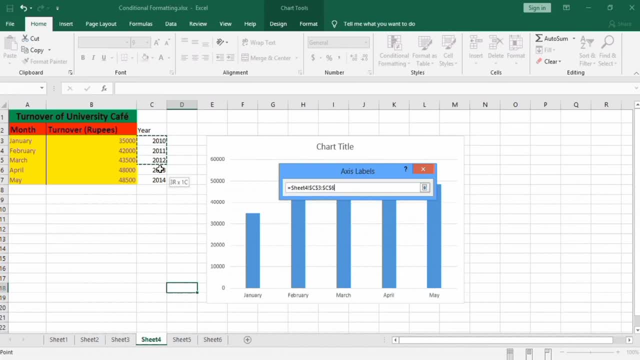 Now I will translate this line chart First show the range of these values. So first I will put h, h next view and adjust the dimensions. Now back to the image selected. now. now click on. ok, now you can see here it displayed years. click again.